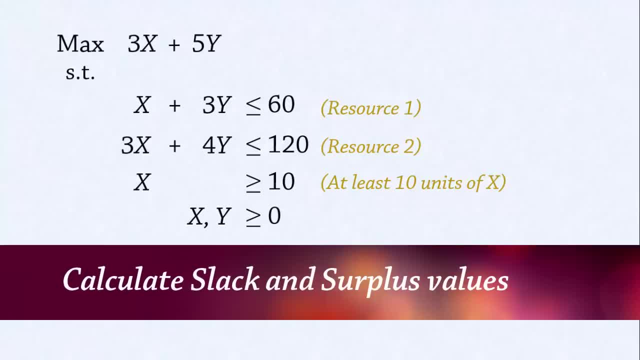 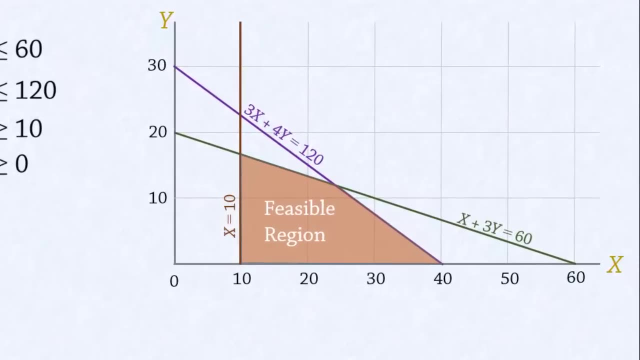 Welcome. In this tutorial we calculate slack and surplus variables, identify binding constraints and write the linear programming model in standard form. Let's begin with this LP model. Here is a graph of the model, showing the constraint line and the feasible region. The optimal solution occurs at the intersection of the first two constraints. 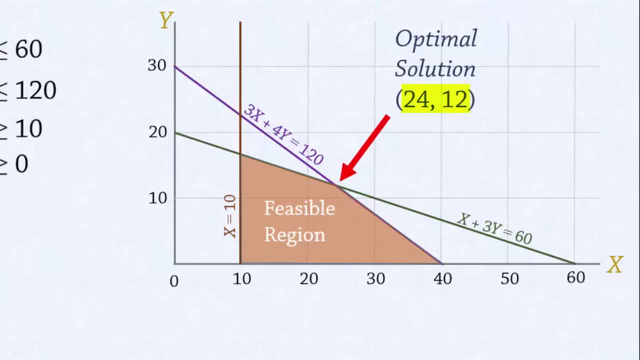 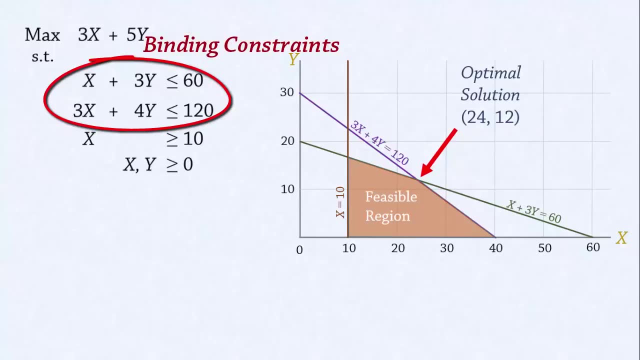 at the point x equals 24 and y equals 12.. The constraints that touch or intersect at the optimal solution point are called binding constraints. So the first two constraints are binding and the third one is non-binding. Now let's see what happens when we plug the 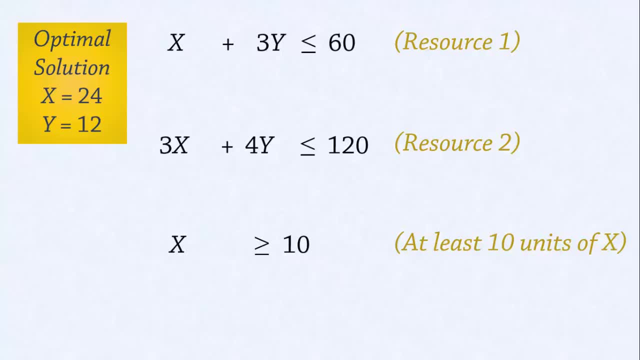 optimal solution point into the left-hand side of each constraint. For resource 1, plugging in x equals 24 and y equals 12 gives 60. So the left side equals the right side. This tells us that resource 1 was fully utilized at optimal solution, That is, there is no slack. 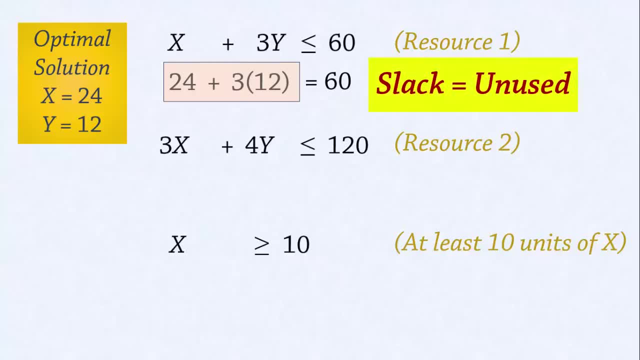 The terms. slack refers to the amount of a resource that is unused and it applies only to less than or equal to constraints. It is basically the amount of underutilization or amount left over. So for this first constraint we have a slack of 0.. That is all the available 60 units were. 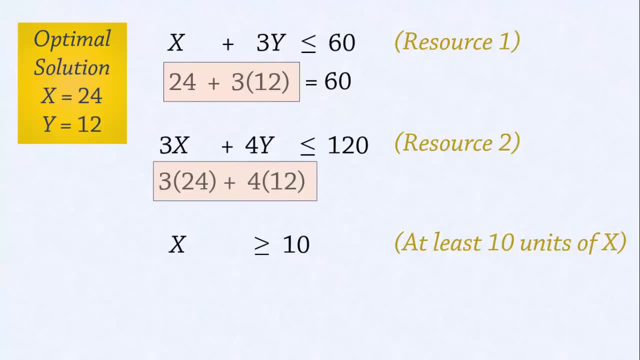 utilized at optimal solution. Plugging the optimal solution into resource 2, we have 120.. That is all available. 120 units of resource 2 were utilized, So we have a slack of 0.. Recall that the first two constraints are binding. It follows that if a less than or equal to 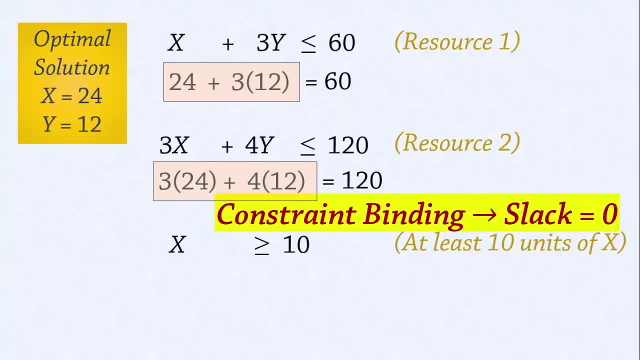 constraint is binding, its slack value will be 0.. The third constraint has a greater than or equal sign. On plugging in x, we have 24 greater or equal to 10.. That is, we are required to produce at least 10 units of x and we produce 24, which is 14 more than 10.. Therefore, because this is a 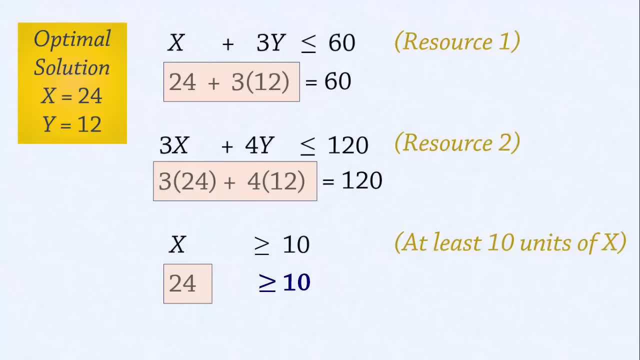 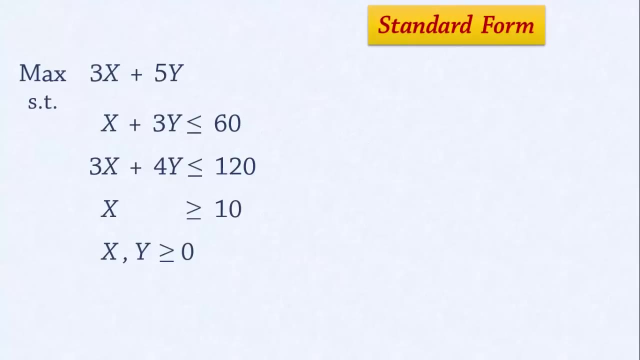 greater than constraint, we will say that we are required to produce at least 10 units of x. We have a surplus of 14.. Suppluse simply refers to the amount by which we exceed the minimum requirement, and it applies only to greater or equal to constraints. Let's now write the LP. 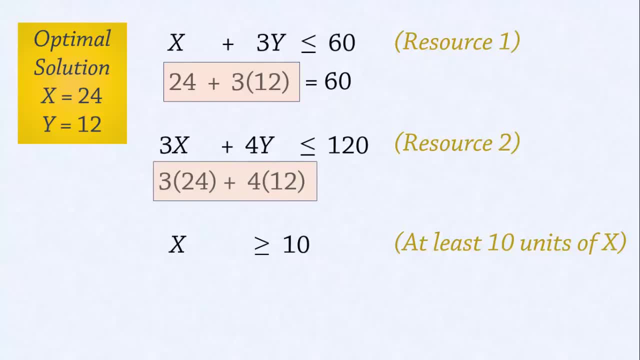 utilized at optimal solution. Plugging the optimal solution into resource 2, we have 120.. That is all available. 120 units of resource 2 were utilized, So we have a slack of 0.. So we have a slack of 0 again. Recall that the first two constraints are binding. 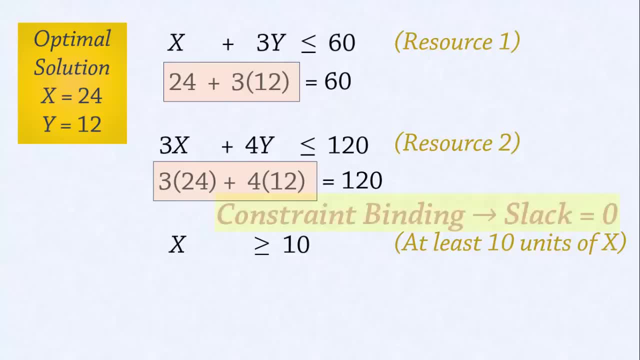 It follows that if a less than or equal to constraint is binding, its slack value will be 0.. The third constraint has a greater than or equal sign. On plugging in x, we have 24 greater or equal to 10.. That is, we are required to produce at least 10 units of x and we produce 24,. 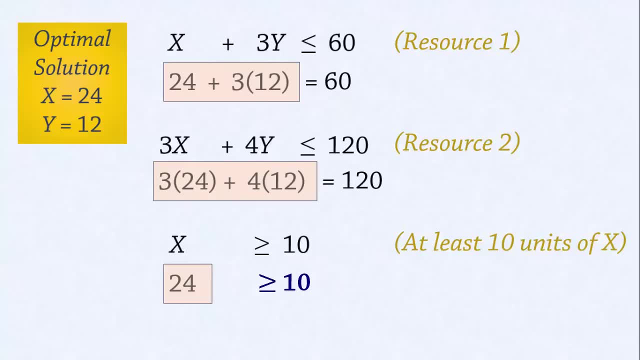 which is 14 more than 10.. Therefore, because this is a greater than constraint, we will say that we have a surplus of 14.. Supplus simply refers to the amount by which we exceed the minimum requirement and it applies only to greater or equal to constraints. 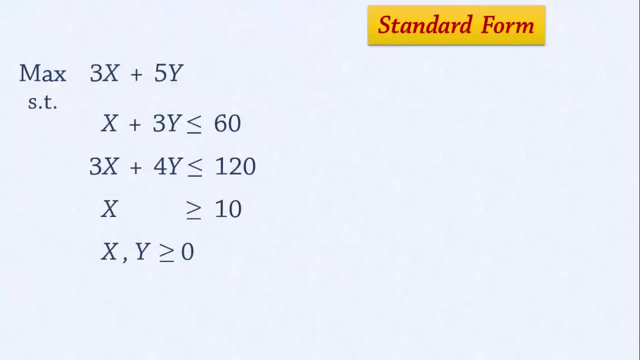 Let's now write the LP in standard form, That is, we convert the inequalities into equalities by adding slack and surplus variables. Since the first constraint is a less than or equal constraint, we introduce a slack variable and add it to the left side of the constraint. 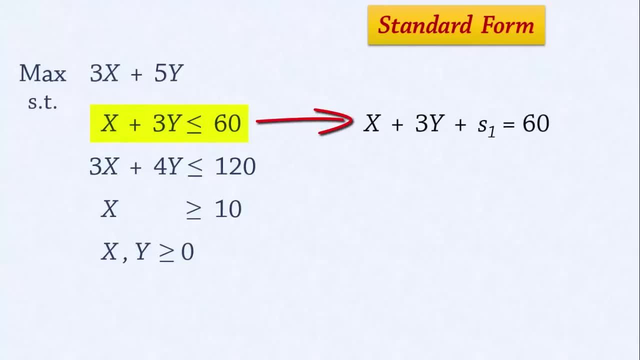 So for the first constraint we write: x plus 3y plus s1 equals 60, where s1 is the slack variable. To write the second constraint in standard form, we add the slack variable s2 and change the less than sign to equal sign, Since the third constraint is a greater or equal constraint. 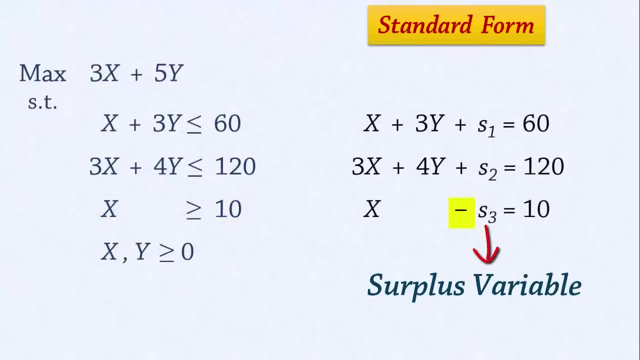 we introduce a surplus variable and subtract it from the left side of the constraint Slack and surplus variables are always nonnegative, So the non negativity constraints are written to include the nonnegativities of the constraints. Now we look at the non-negativities of the constraints, which are written to include the 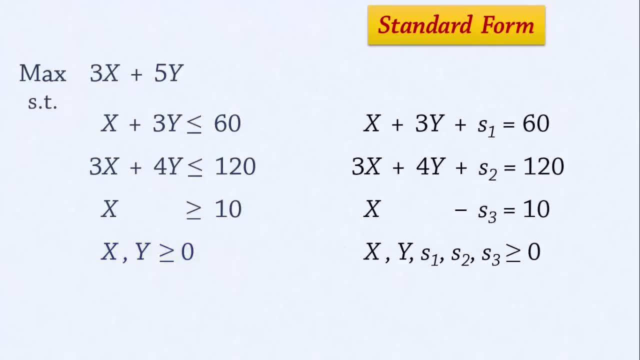 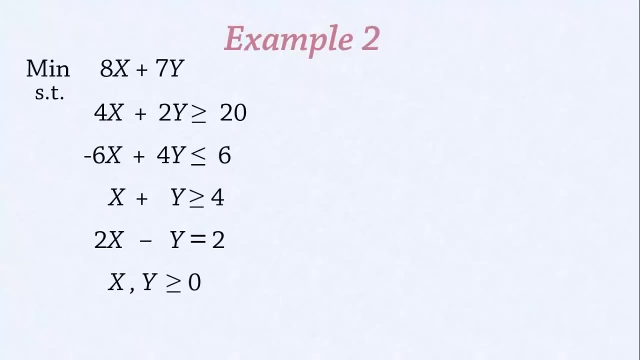 slack and surplus variables. The slack and surplus variables do not affect the objective function in any way, so we usually just include them in the objective function with zero coefficients. The standard form of the LP is now complete. Let's see another example. Suppose the optimal. 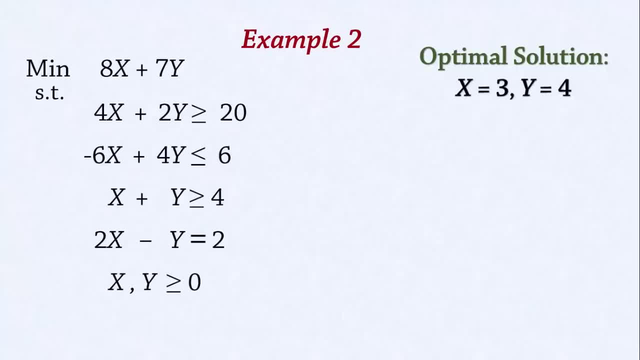 solution to this LP model occurs at x equals 3 and y equals 4.. We want to write it in standard form, calculate the slack and surplus values and determine which constraints are binding. Let's first write it in standard form: The first constraint as a greater or equal sign. 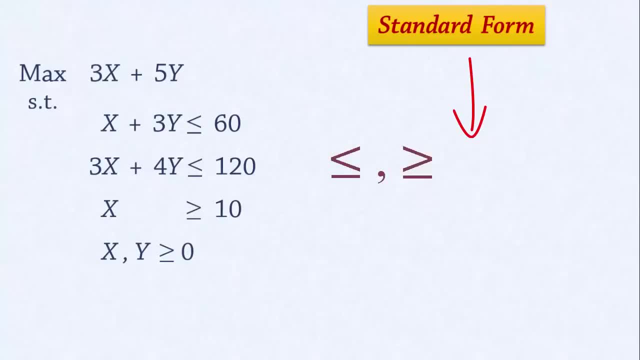 in standard form, That is, we convert the inequalities into equalities by adding slack and surplus variables. Since the first constraint is a less than or equal constraint, we introduce a slack variable and add it to the left side of the constraint. So for the first constraint, 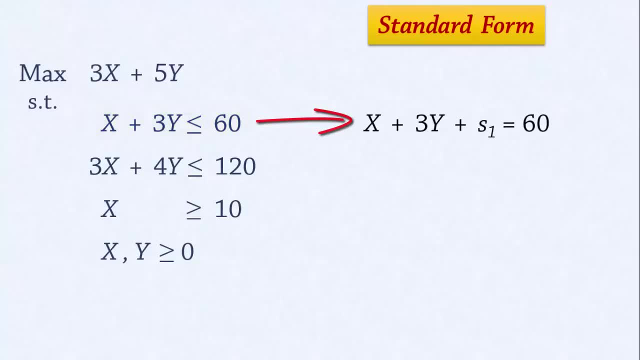 we write: x plus 3y plus s1 equals 60, where s1 is the slack variable. To write the second constraint in standard form, we add the slack variable s2 and change the less than sign to equal sign. Since the third constraint is a greater or equal constraint, we introduce a surplus variable. 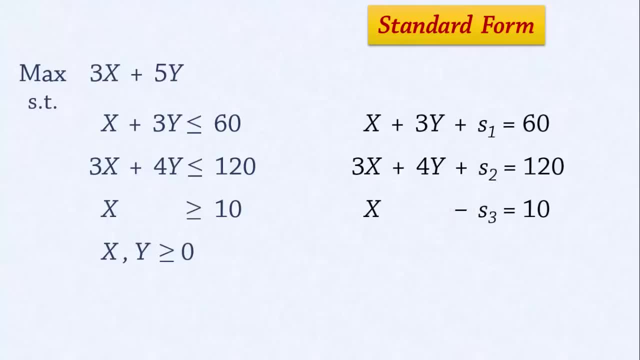 and subtract it from the left side of the constraint. Now slack and surplus variables are always non-negative, So the non-negativity constraints are written to include the slack and surplus variables. The slack and surplus variables do not affect the objective function in any way, So we usually just include them in the objective function with zero. 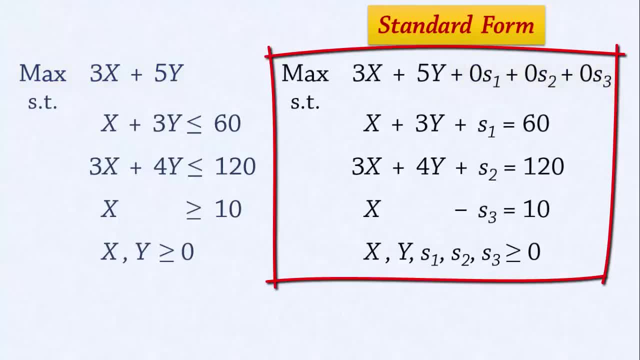 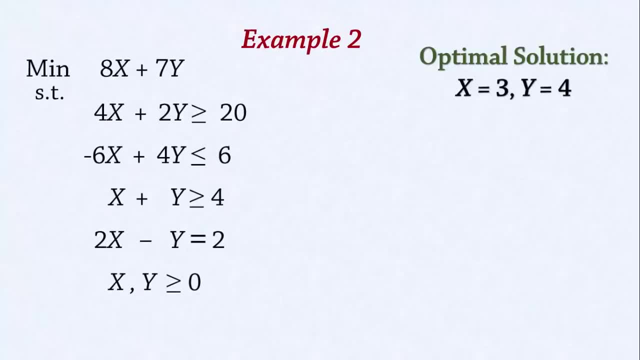 coefficients. The standard form of the LP is now complete. Let's see another example. Suppose the optimal solution to this LP model occurs at x equals 3 and y equals 4.. We want to write it in standard form, calculate the slack and surplus values and determine which constraints 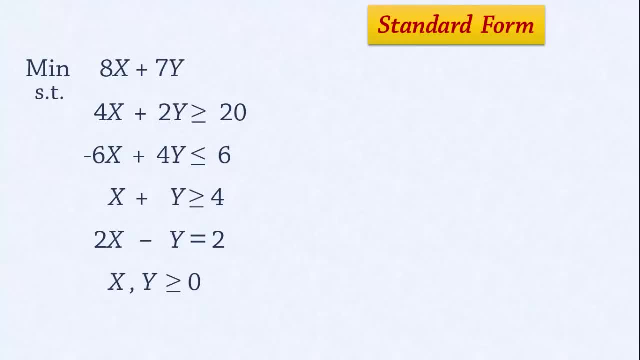 are binding. Let's first write it in standard form. The first constraint has a greater or equal sign, So we introduce a surplus variable with a negative sign as we convert the inequality to equality. The second constraint has a less or equal sign, So we introduce a slack variable with 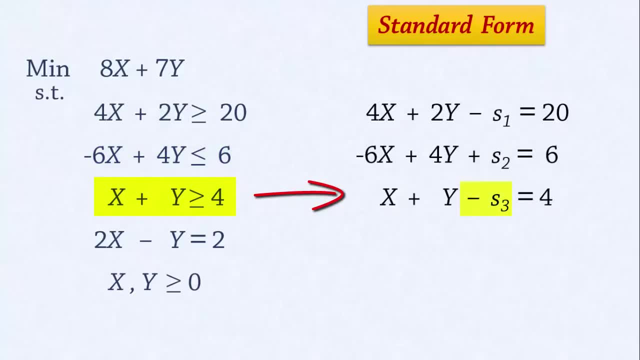 a positive sign, The third constraint will also have a surplus with a negative sign. The fourth constraint is an equality constraint. Since the purpose of writing the model in standard form is to convert inequalities to equalities, this constraint is already in standard form because it contains equality already, So no slack or surplus variable is. 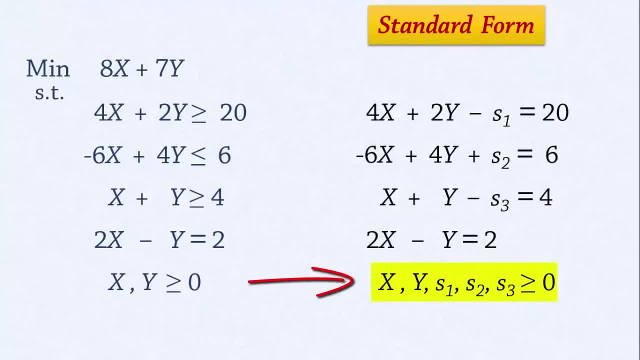 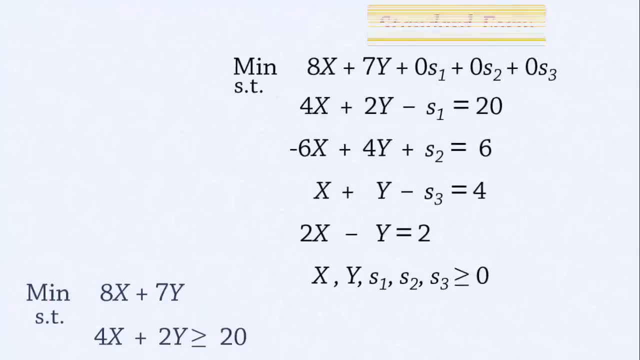 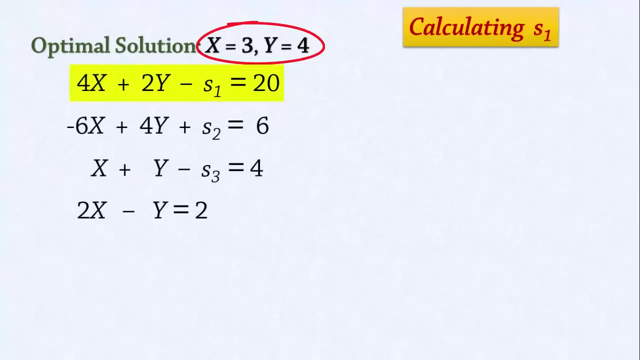 needed for this fourth constraint. Here are the non-negativity constraints and here is the objective function. We now use the standard form of the constraints to obtain their slack and surplus values. Recall that the optimal solution is x equals 3 and y equals 4.. So for the first constraint,